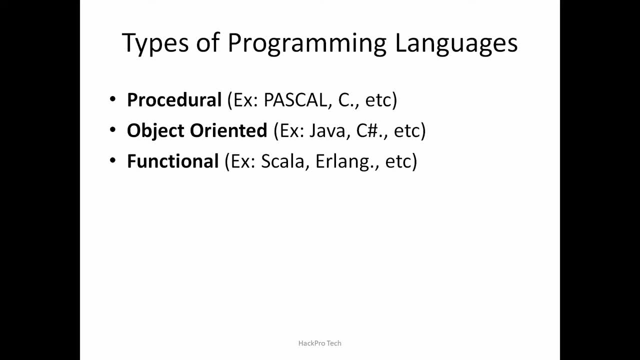 object oriented is a bit different. so, for example, c plus plus and java, those are the object oriented programming language. so because here we're going to deal with completely with objects, each object going to relate with the entity, so, um, it's not kind of a sequential. so because you have one, 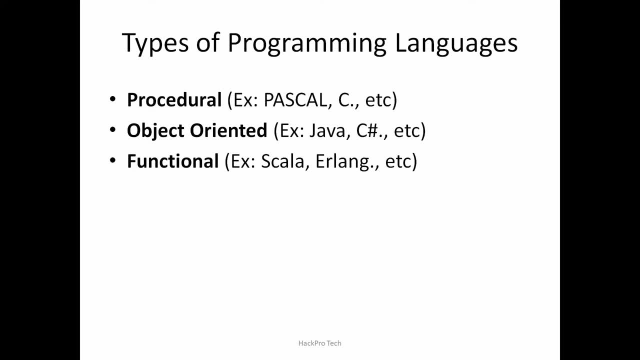 object with another object, for example, you have the person object, person class, though that going to represent one particular entity, right? so that is where this object oriented comes into place. i mean comes into picture. okay, so now you have a question, so procedural and object oriented is fine. 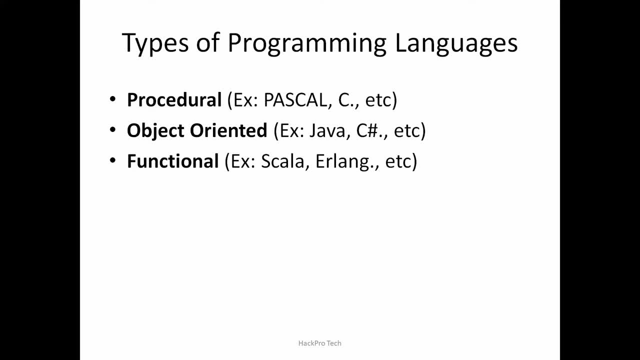 but what is the functional programming? functional programming, i would say, it's a, it's a kind of a fun. i mean programming style, i mean coding styles. that that is, that is the one thing i can tell you, because, um, you can, you can reduce a lot of codes, um, a lot of codes, and, uh, one one, one key, i mean one. 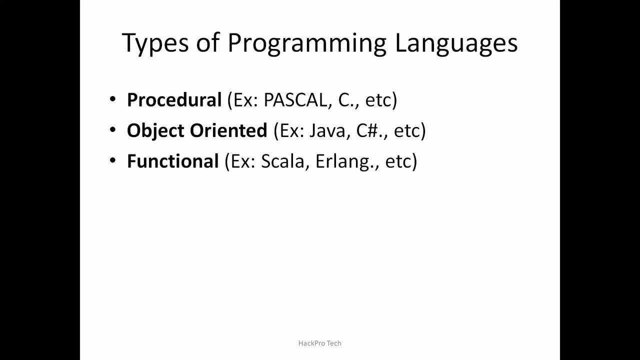 phrase, people will totally get confused. i'll tell you that phrase okay, function is a first class of first class object. so this is hard to understand. okay, i know it's hard to understand, but the thing is it's simple. so before that you have to understand that what is the first class object? 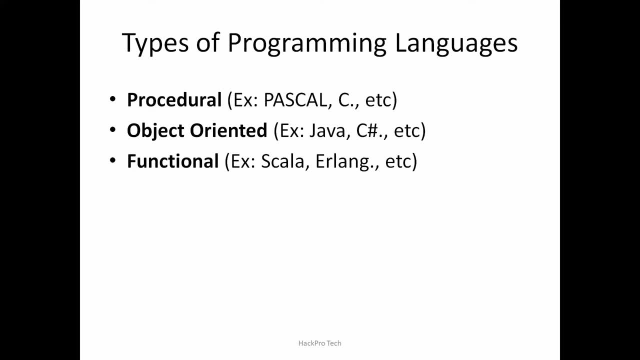 first class object in the sense it's a value. whatever the value, are telling that those are the first class objects. okay. so if you try to treat function as a first class object, then so then then that that that is what they are trying to say: function is a first class object. okay. so here um functional programming. 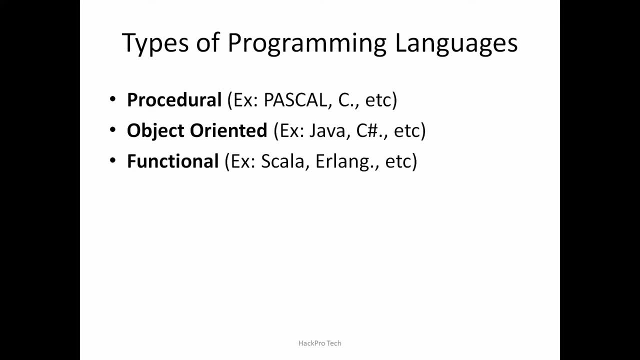 scala airline. those are the. those are the language with support for the functional programming um. so still, even though java is object oriented, after java 1.8, java also tried to support um functional programming. okay, using streams, api, they are supporting the functional programming. so still, you can able to act you in the java, okay. 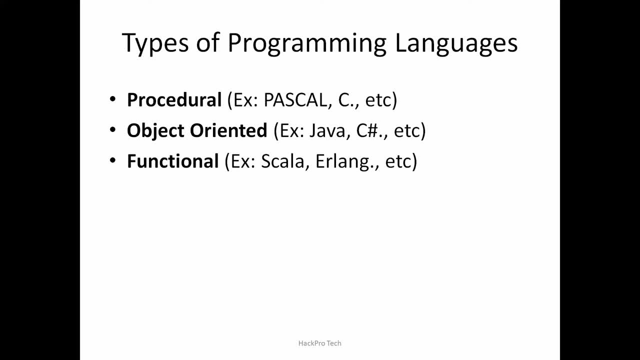 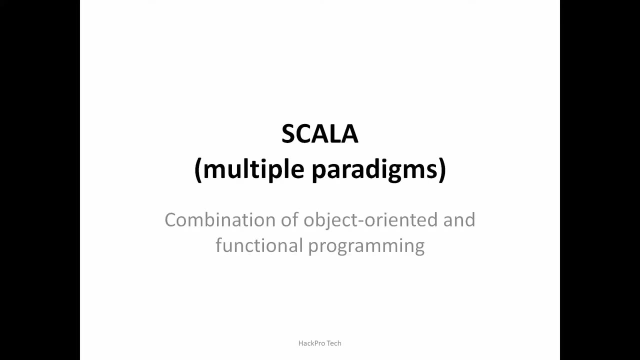 after 1.8. um, but the thing is here. you have to understand one thing: scala is written on top of the java, okay. so so scala also use java, usually use the jvm, right? so whatever the codes you are writing, so those codes can well. i 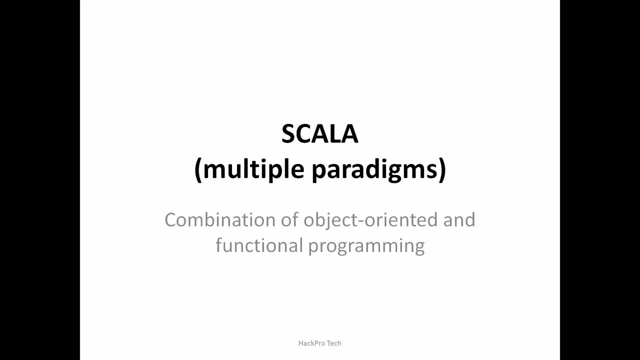 mean those codes going to be converted into byte codes, those byte codes going to run it in the java java virtual machine, right? so same process going to happen in the scala also. scala also going to convert into the byte, byte code and byte code only going to run it in the java virtual machine. 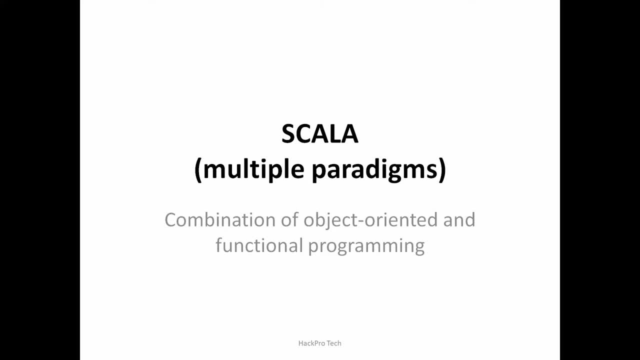 but the thing is because scala also written written on top of the java right. so scala will provide the functional programming as well as the object oriented in the very elegant way. okay, so, um, don't get cut, don't get confused. i will explain the. uh, i will explain all those things in the deep. 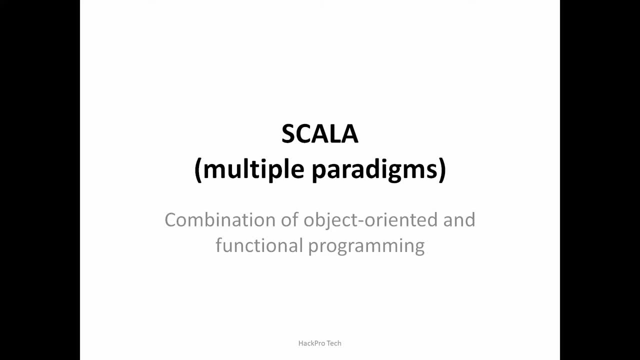 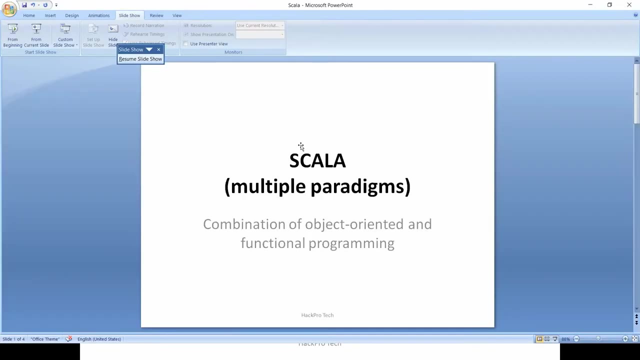 but this is where this functional programming will come into picture. okay, i'll, before i will go go into the further things, i will explain one small things. with the- uh, that particular phrase, four hunks are not treated as a first class object. okay, let me show you something. 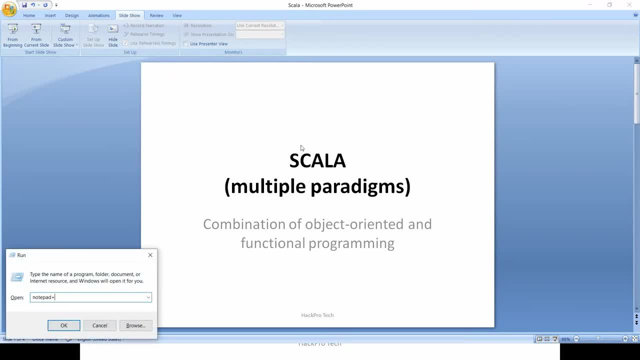 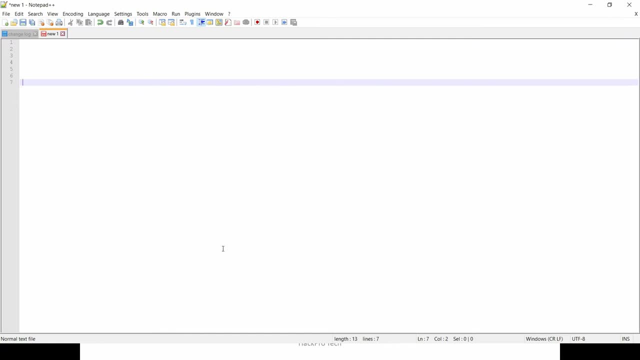 okay, i'll open the notepad plus, plus as of now. okay, so, for example, if you're typing val, this is a declaration. okay, declaration of i'm declaring one variable. okay, don't can get confused with the syntax, whatever i'm writing, just imagine i'm declaring one variable, um variable like um name. 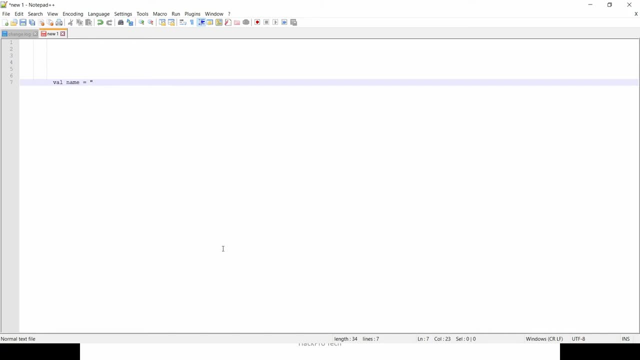 and i'm giving the value of hack pro. okay, so i i already mentioned that, whichever the value you are telling, those are the first class object, right? so here, name equal to hack pro. so that means that this is the value. it's a value of string, so this will be considered as a. 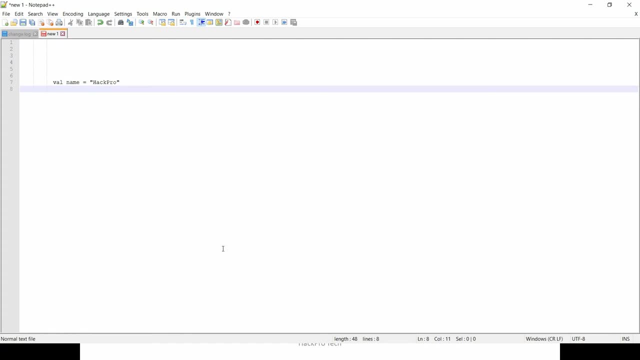 first class object, right, but this can be achieved in any languages, right. but if i tell you val um, for example, name function equal to function, if I declare like this: is it possible, is it possible to act? you just imagine in that way? okay, because you cannot, you can't. 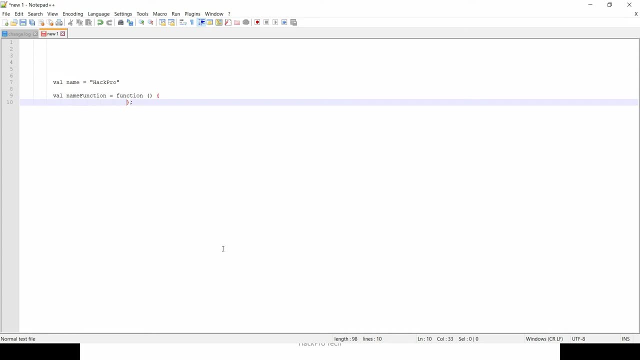 able to declare the function as a value. right, so, but this is the core thing for the functional programming. you can treat function as a value, then you can pass this. I mean, if you treat the function as a value in the sense you can pass this as an argument to any of the functions, right, any of the function functions. and 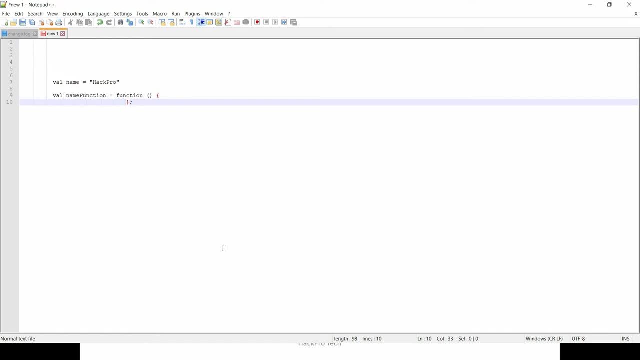 you can pass anywhere, so you can play around with that, right? so that is where this particular phrase will come into picture. functions are treated as a first-class object. okay, now I, I think you might, you might clear, okay, okay, let's, let's move on to the next thing. so. 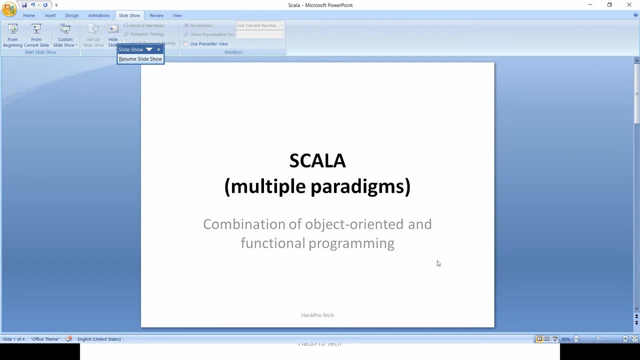 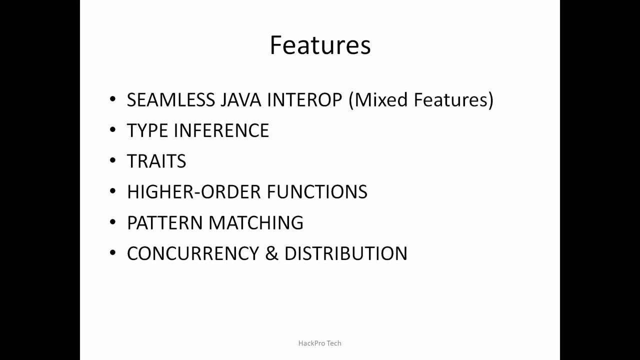 that is where this Scala will come into picture. so Scala, if you see, it's a multi paradigms. that means it going to support for object oriented as well, object oriented and functional programming as well. okay, so I'll move on to the next thing. see what are the features Scala is providing. okay, first, 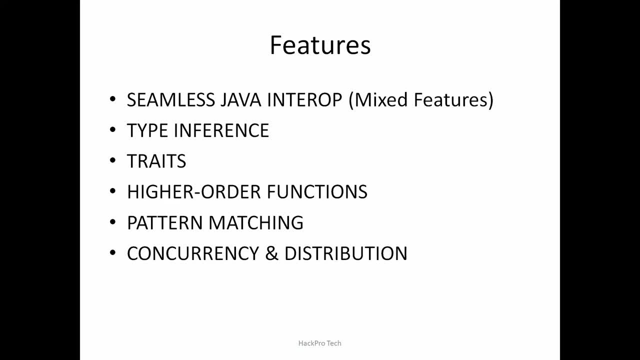 thing. these are the six features. I mean this is a high level. I am going to explain, but in further videos we go. I am going to explain the depth. what are the exact feature? I am going to explain the code also, don't worry about that. only basic, basic concepts. I am going to explain the slides. okay, so now we can. 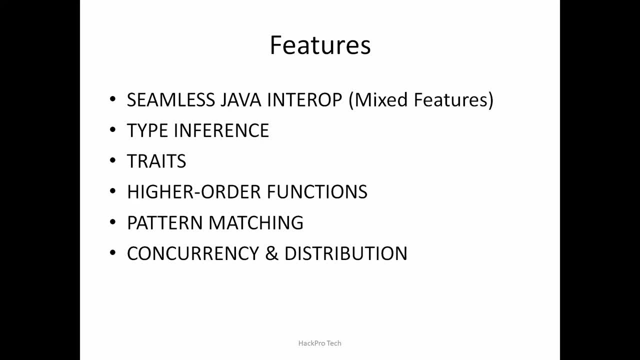 see seamless Java interoperability. okay, this is that. I already explained that Scala is written on top of the Java, right, so done means color also going to is the same JVM. so if you take one project, that project, you can write some Scala code along with the Java code also. both will. 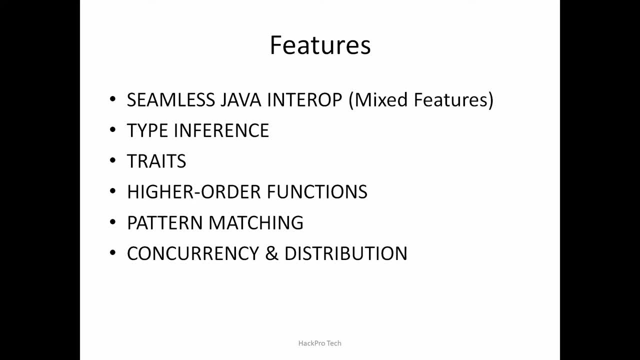 work you can. you can use the both the things. that means it is a mixed feature, right, because both the course going to convert into the bytecode and both the course, both bytecode can be run, run it in the Java virtual machine so so that in particular language might mix the feature. you can able to act, you, that is. 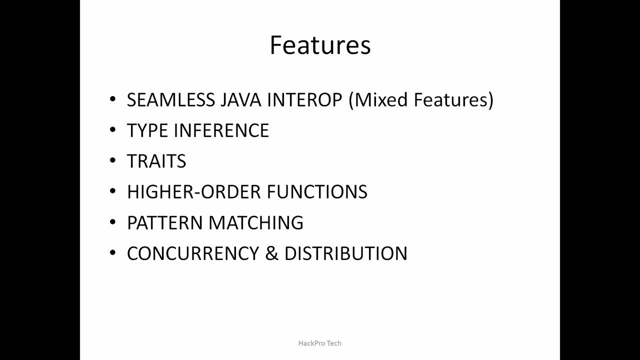 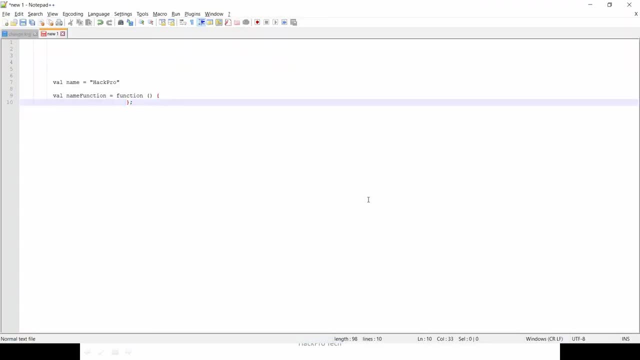 the first thing. second thing is that type inference. so one thing you might notice I have already shown in the notepad also. okay, let me open this one. so usually how you will declare on particular variable, okay, so for example, you will declare the variable like public string. mmm, I can give a mark. 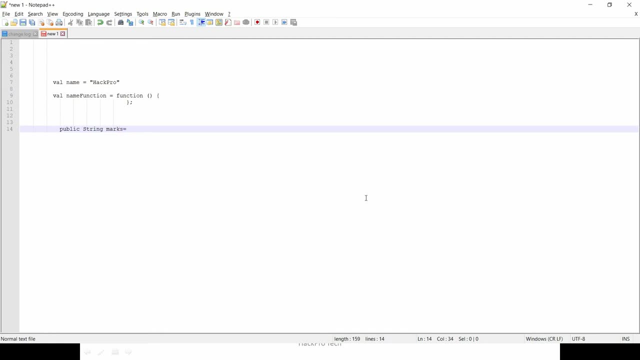 marks. so not, okay, not marks can give first name, first name, hack Pro. okay, so this is the variable that we are going to declare on particular variable. okay, so, for example, declaration right in the Java: okay, I'm, took the job as a example. okay, here, if I? 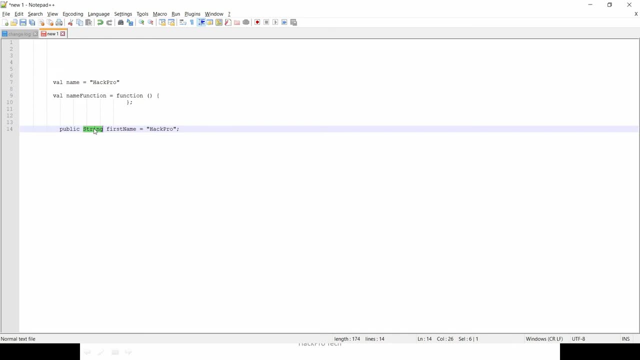 remove this one, if I remove this string, what will happen? the compiler compile time itself. you will get a error because it can't able to compile. there is no type definition for this particular variable, right? so? but if you take the same example in this color, okay, I'll return like this: okay, well, first name. 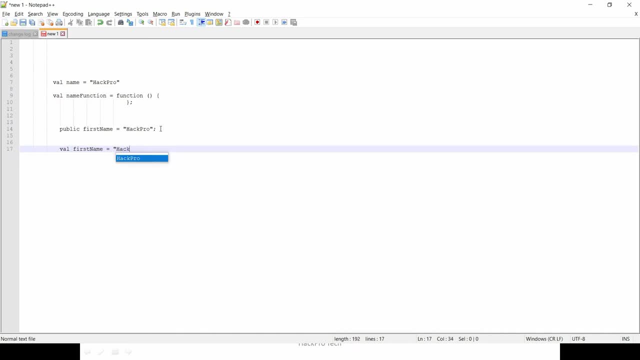 is equal to hack Pro. okay, so same thing. I have written here, but without. I'll just place it here because of the confusion. okay, this place is the string over there. okay, this is Java. this is for Java. this is for Scala. it's first color. okay, so in this color and the variable declaration, I haven't 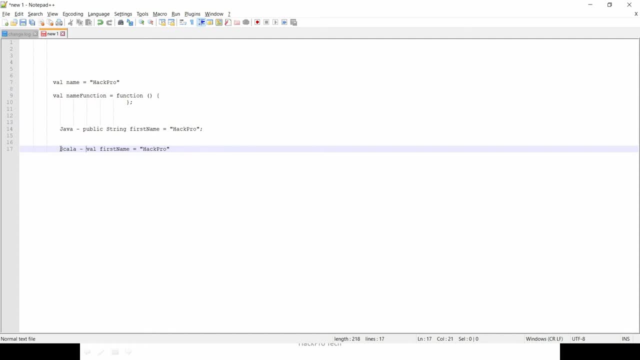 mentioned any places, the string, the type I haven't mentioned, but still you can mention. but there is no type definition, right? so yeah, I mean the above one is the type system. you have to give the exact type, then only it will take, otherwise it won't take. okay, but if you take in the Scala, there is no type. 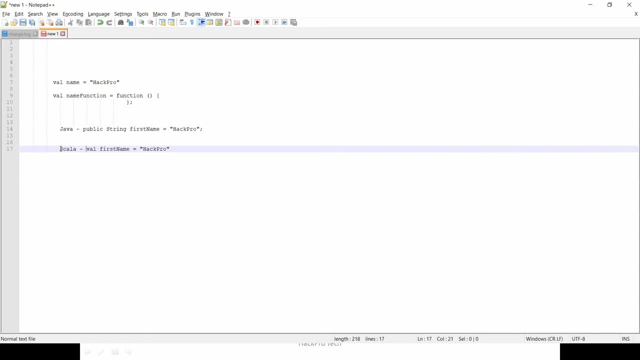 definition here, but the compiler will automatically decide with the value. whatever the value in the right-hand side it will consider: okay, this is the type for the particular variable. for example, here, if you see, has hack Pro is the value I'm given right, which is in the enclosed door, I mean. 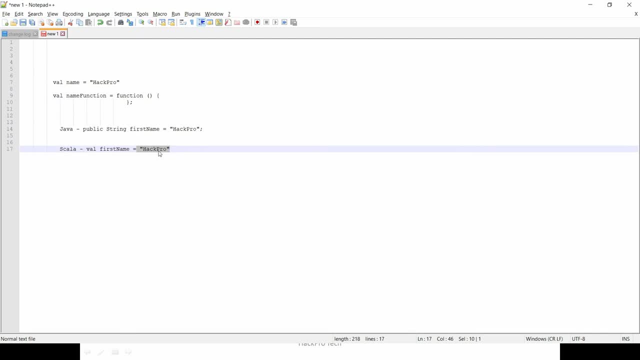 double quotes. so that means this is a string. so automatically can compiler we infer the, infer the type, which is I mean for the type of a string, because based on this value you're going to, I mean assume that, okay, this first name will be the type, first name type will be the string. okay, so then the final, if you're. 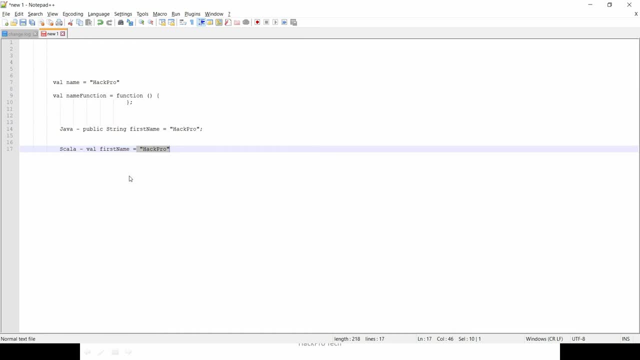 trying to print this one, so it will print as a string. okay, if you hover also, you will get that, but I will show you it in the ID itself. okay, so this is the type function and other things you can do in here in the. but in the Java you can also try to give this type of a string for this type of a. 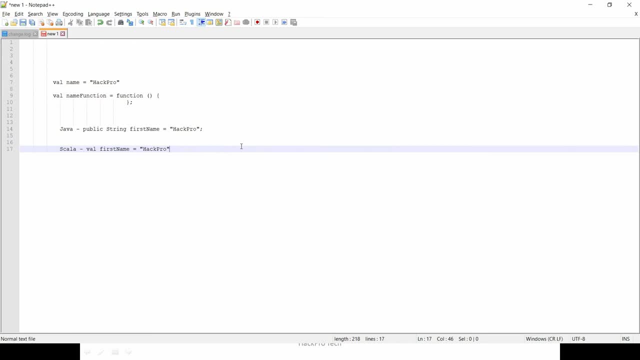 string. okay, so you can see the type of a string. you just need to enter the type to be happy. and also the sign name of the type of a string goes into the strata which is in the top left-hand corner. so that means that the whole 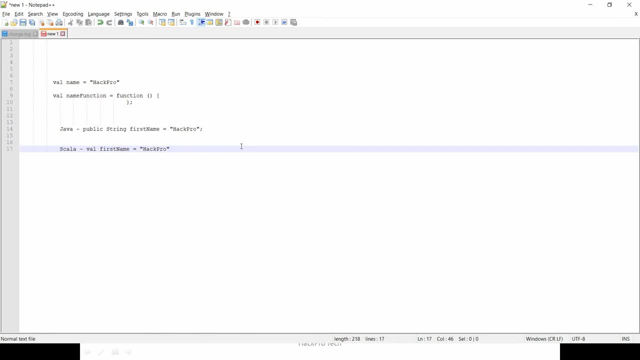 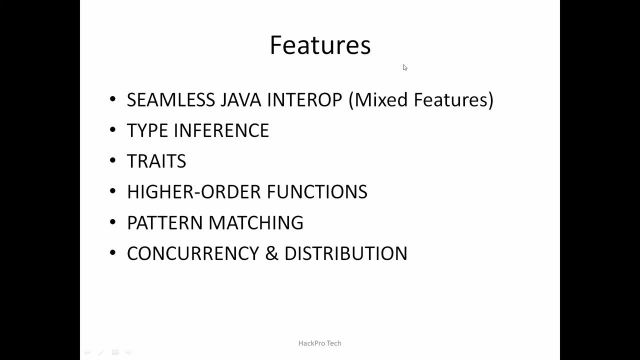 thing is called a type expression. okay, now just understand the concept. first programming. you might see some different, different things. right? this is the first thing. okay, this is what i told you in the function. i mean, uh, this type inference. okay. third thing is: trites, trites. 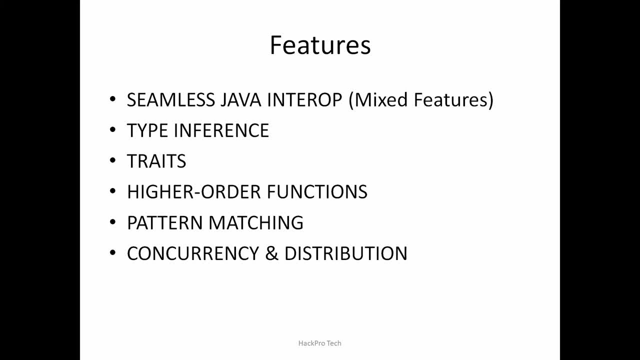 um you in the java, i, i will, come, i will. most of the time i'm going to compare the java only. okay, if you are a dotnet programmer, you just compare um, uh with the dotnet thing, but the java, because scholar also written in the java, right? so that's why i'm going to compare some, some. most of the 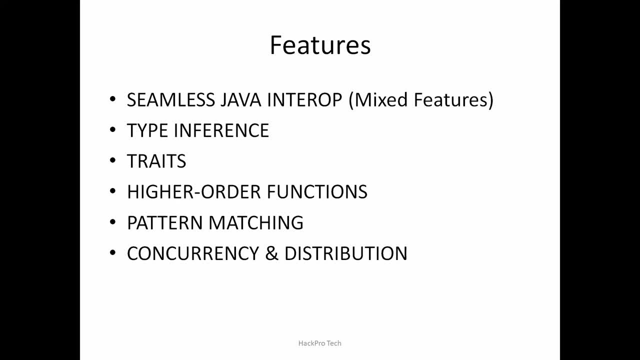 things with the java. only just to think about that. um, just try to relate such things. okay, i'm going to give it in the high level, only i'm going. i'm not going to, uh, give any complex things. um, the thing is trites. in java there is a things like classes and interfaces, such kind of things. right, 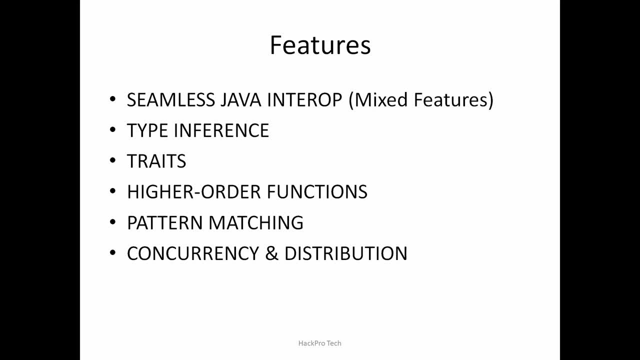 so those things we can actually, i choose, i mean we can same thing we can actually in the scholar, also using the strides. try it: if you directly compare with the java, you can compare the interface. okay, you can to actually, uh, multiple inter interface using the sorry, multiple inheritance, using the traits, okay. 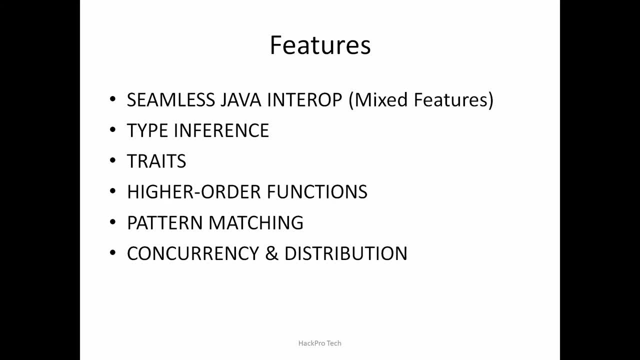 and the fourth thing is higher, higher order function. so you um, in the beginning of the video i told you the function is treated as a first class object right in the higher order function. you will, you will mostly see these things okay, because you will assign some um variable with the function as a value and you will pass this variable. 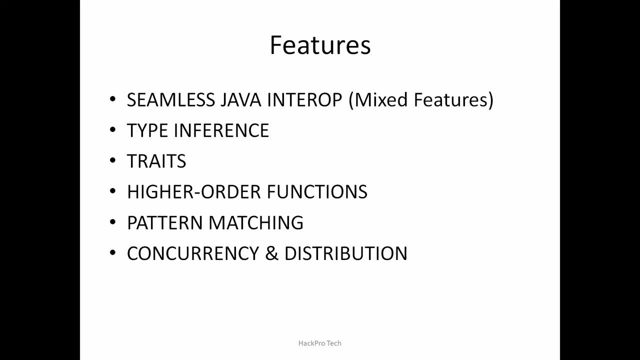 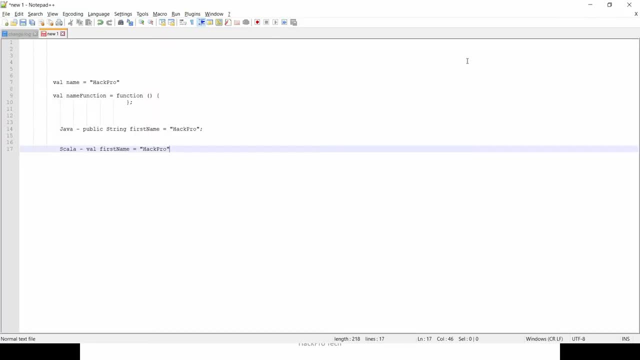 to the another, another function, and that function will return the uh, return the another function. okay, so i i will tell you, okay, for example, so this is the name function, right, this is the name function i have written. so now, if you take, um, so, if you take, i'm going to uh, define one function. okay, uh, this is the function, function one. 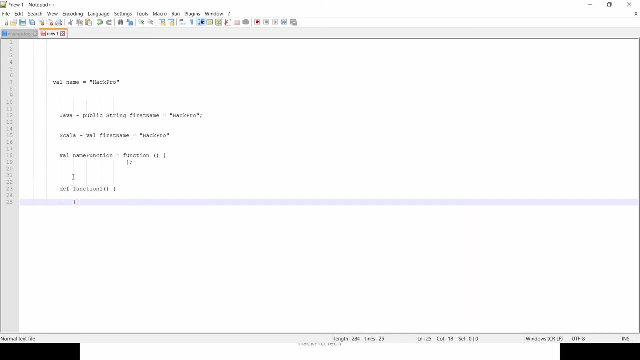 so it going to return something. i'm going to return, return something. just imagine: okay, it's not the exact value, i'm just writing the pseudo code. okay, um, written something. so if i pass this name function because this is a value, right, so then directly i can pass this as an argument to this function. right, so i i can declare function. 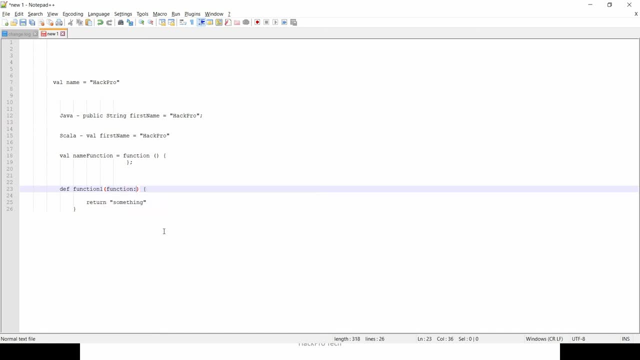 is a function object. okay, so if i invoke this function, for example, if i try to invoke this function, what i will do? function 1: name function. so you you can able to understand right, so this is the function. i mean normal function definition i given. so i have already declared one function. 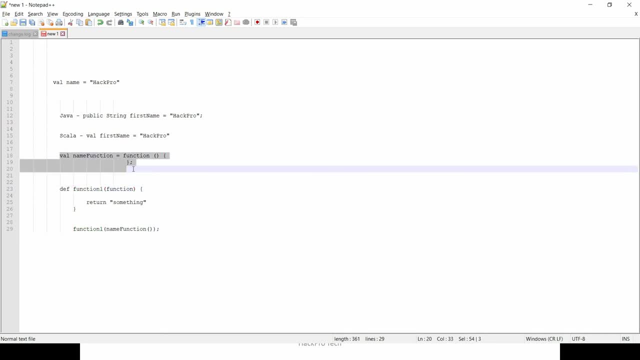 as i i mean function. i've given the function as a value to the name function and just. it is a function, of which three questions are given. and one of the question is: it is a function of two actions. right, just passing the um, this particular name function into the function as a argument. right here is the. 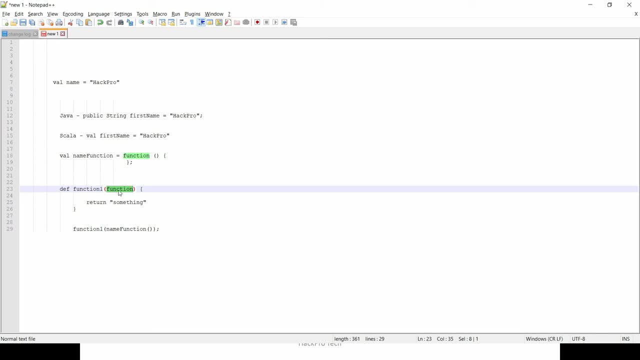 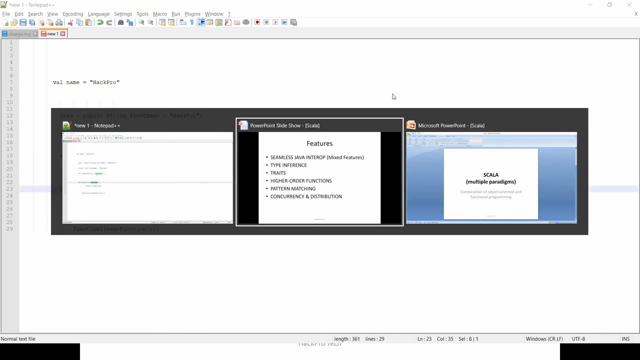 parameter. if you see function, so this is what the higher order function will come. so i will explain it deep. but this is where the higher order i mean higher order function. so if you're trying to pass uh as an argument or the function also going to return the return another function, so that that 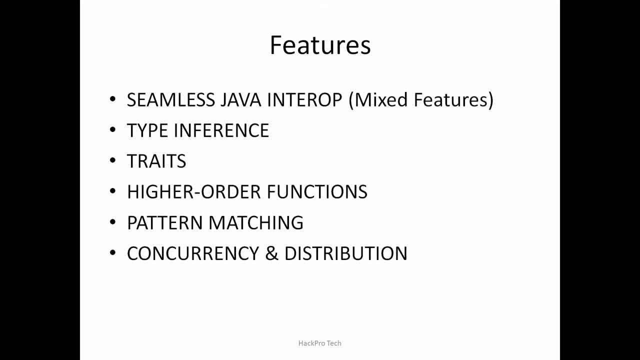 is the- that is the thing. higher order function will come into picture. okay, uh, pattern matching. pattern matching is one of the- uh, i mean very good feature in scala. so, um, if you directly compare with java, so it's like kind of switch statement. okay, uh, don't think it's a switch. 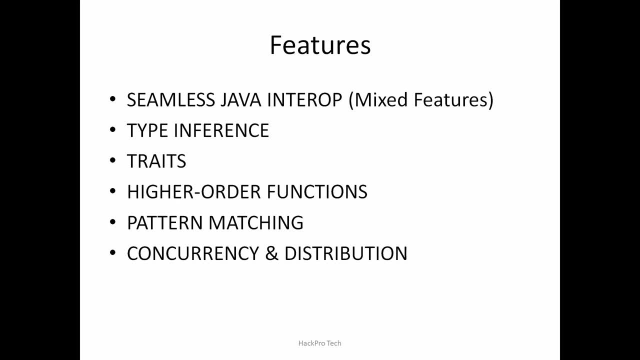 statement, but it's kind of switch statement. you will get more features, benefits from over there, okay, so i will explain in deep, okay, and concurrency and distribution. so this will uh, this is the advanced things. so this will comes into the reactive programming like, uh, asynchronous programming. you will hear that, uh, i mean whenever if you're trying to. 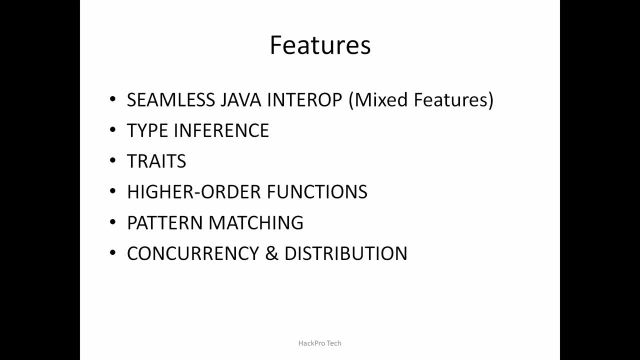 processing, some parallel process. uh, do some parallel processing over the collections. so then, uh, the concurrent and distribution will come into picture. so you people might hear about few futures. futures, uh, with the asynchronous programming, those also will come. so, like you will hear some uh framework, like aka actors, so those keywords you might hear, uh, if you're not, 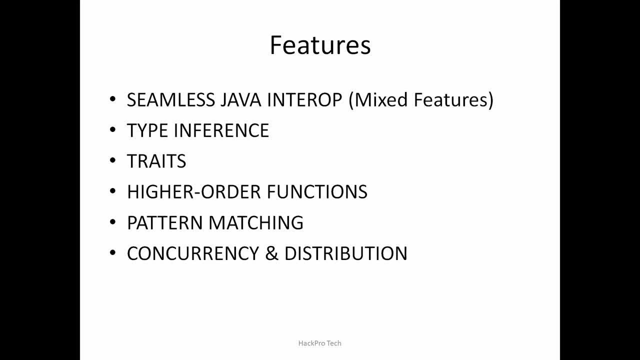 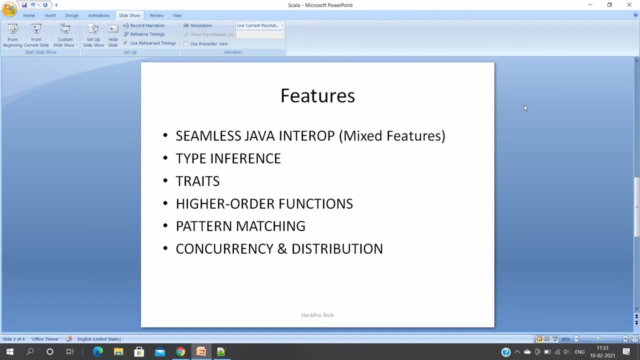 familiar with that. i will explain in deep. okay, so this, i mean, is a asynchronous program. if you're trying to do that, that those will comes into the concurrency and distribution things. okay, so these are the features which is offered by the scala um. so this color programming language, you people 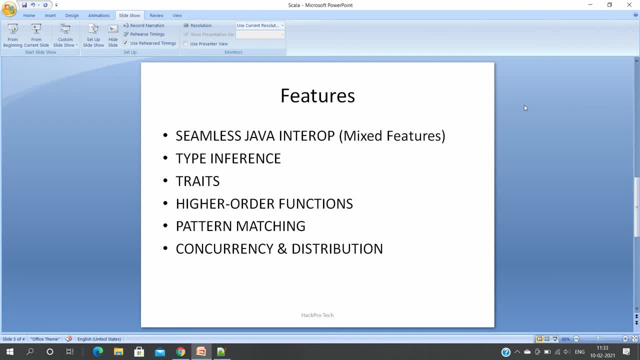 might will think, okay, where they are exactly using, because there are a lot of languages out there, even python's, uh, javanet scholars, though, so many languages are there. so where exactly they are using actually, um, some, um, application development. okay, scholar might i mean uh, java might will, uh might. 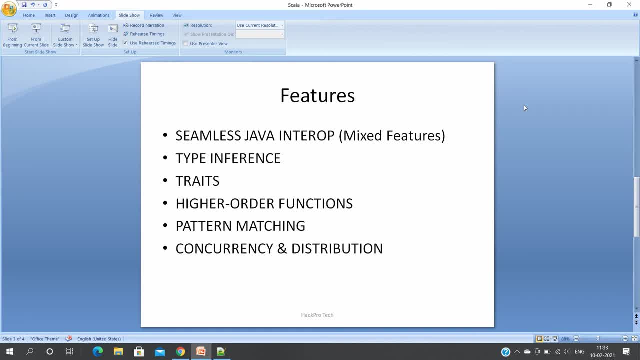 be the good option. okay, but when we, when, if you go for some other tech stack like big data, those stuffs, okay, machine learning scholar plays a very- i mean, major role. okay, because, um, here in the functional programming, the, whatever the code you're writing, it's very less when compared to the. 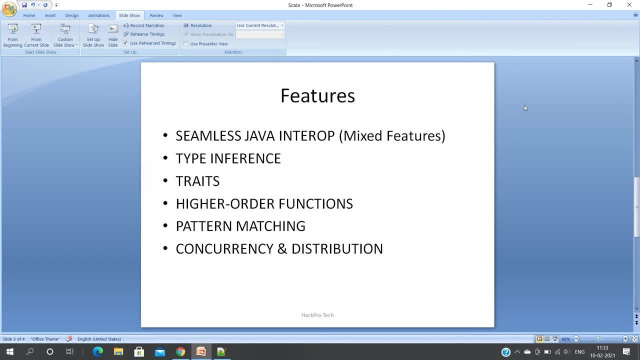 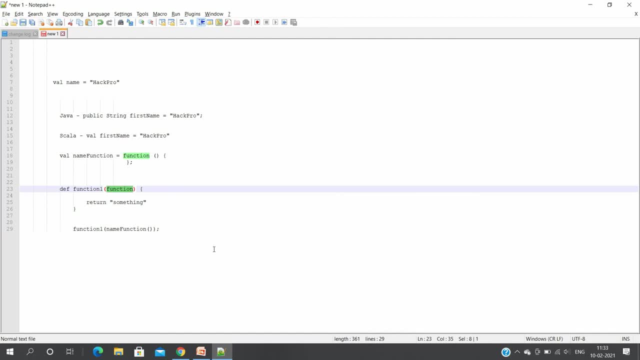 um, i mean other languages. okay, i will tell you one important thing. okay, you will. you will see, um people will tell: okay, you will. uh, there is, i mean um, you won't write much code. you won't write much code. that particular word you will hear, i mean this particular sentence. you will hear it from many of the people that means: 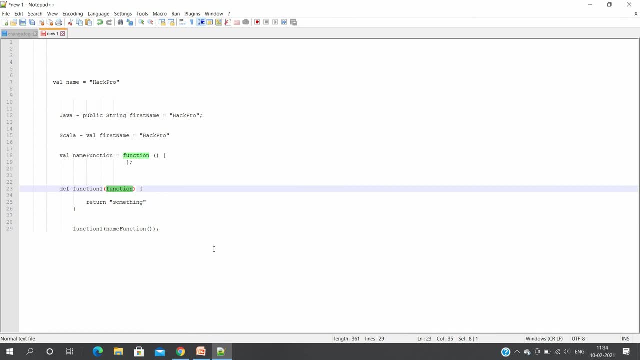 here the brevity will be. i mean, the scholar will give the brevity. okay, because you can write same, same things, um, um, in a very short, short manner. okay, for example, if i am trying to do, uh, some operation over the collections, okay, uh, i have list of students, okay, i'll, i'll tell you. 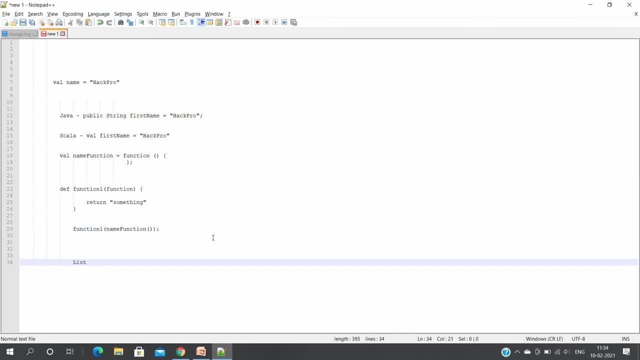 okay, i have a list of students. um, okay, list of students, or example, or else the list of string i'm give. okay, i will keep the list of string. so here, if you see, um, i'm going to don't get confused with the syntax, i'm just giving the pseudo code, okay, um, it's like i'm going to do. 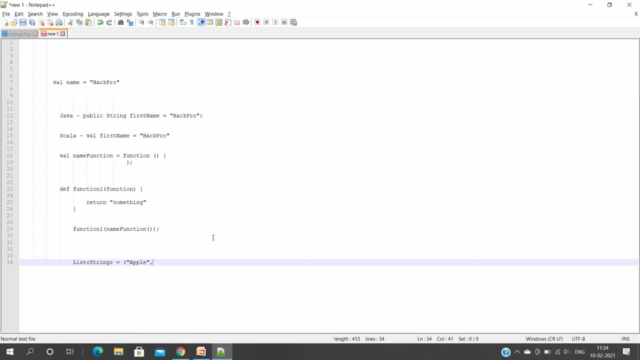 the same thing. but i'm taking some fruits. okay, apple, orange and pineapple. okay. so these are the fruits, are there? okay? so what i'm going to do, i'm going to take, pick one particular fruit, okay, uh, in the, if java is a verbose language, some people will tell because 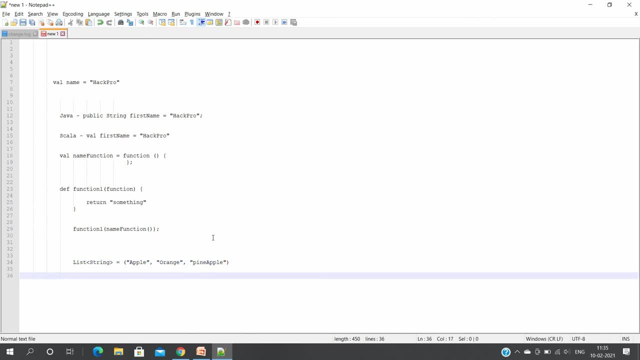 you have to write many, many lines of code. i'll tell you why this is laziness. so if i'm going to do this, uh, i mean i'm going to filter only particular fruit. i mean only two fruits, okay, apple and orange. i don't want the pineapple fruit, uh, fruit what you. 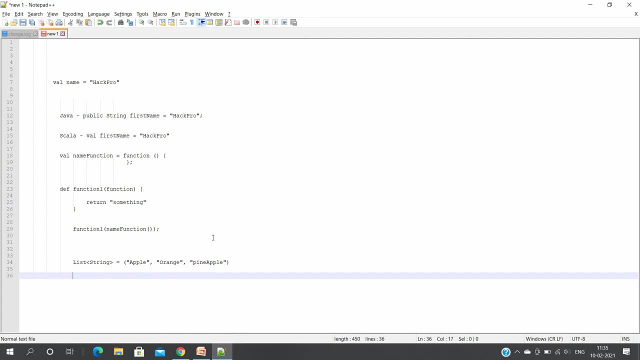 will you, people will do so. you have to iterate. obviously you have to iterate using forage, enhanced forage, kind of things people do- and you will do iterate and you will put it in some other- uh, or i mean- list and you will return the results. right, this is the way- our traditional, i mean. 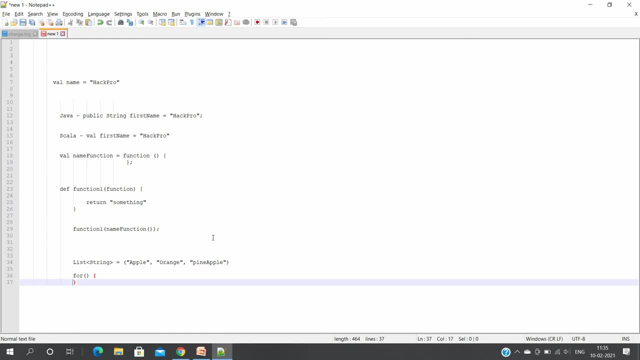 imperative language will come into picture. but the thing is, when you come to the previous time, there is also a kind of word Kin, pencil machine or some other thing that are used in order for you to use exactly this method. right, if i am going to do this, i'm 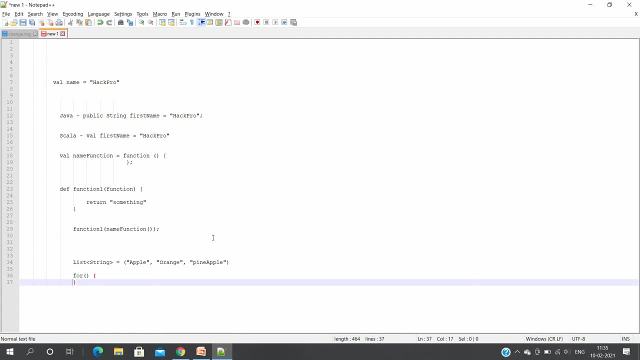 to functional programming. you can do these steps within single line, right? you can avoid multiple lines of code. that is where this- uh, i mean limit, i mean limited course- you will write. there's a brevity in the code. those things will come into picture. and one more important thing you will get: 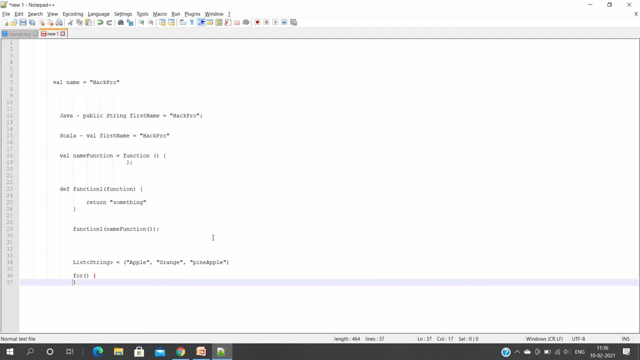 um, one word. it's like what to do, how to do? okay, the thing is what to do, how to do in the sense, this is what we're going to. i mean, our objective is we're going to filter only orange apple, those fruits. right, that is our objective. that is what, what, what we are going to do? and, um, i 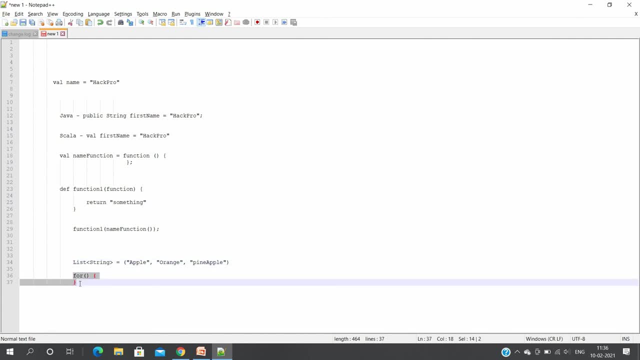 mean how to do in the sense we're going to implement- right, we're going to implement- the forage loop, then we need to hydrate each uh items in the list and we're going to said, i mean, we're going to put it in the separate list. this is what we. i mean this is the how to do, but when? when? this. 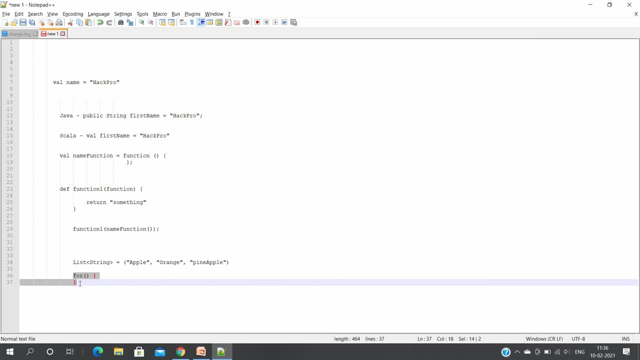 comes into the functional programming, you will see: um, only you need to focus on the what to do. that means you, you, you can focus directly on: okay, we need to filter only i mean apple and orange. okay, we, we don't need, uh, the pineapple, that means we need not to write. i trade this entire list and we need to filter such things. we can do it in the 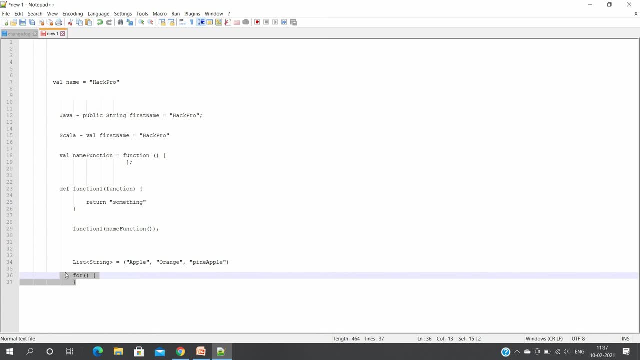 uh, predefined functional functions. okay, there are a lot of stuff. i will explain by one. okay, um, as of now, i hope i'm going to um, stop over here, because there are a lot of things we're going to see, um, but these are the basic things. when you come to the functional programming, 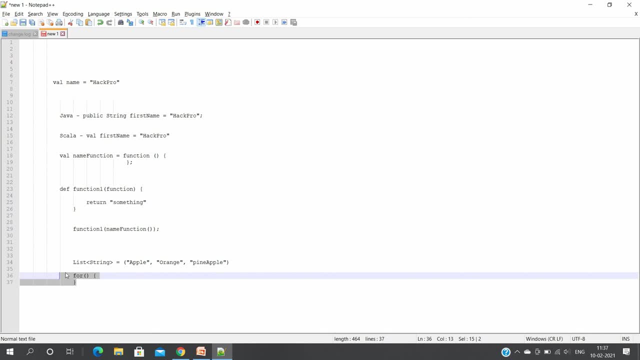 i i already given the example of where we are using this scala in. i mean real time scala. we are using in the big data stuff. so machine learning over there we are people widely used. okay, uh, still, uh, you can use the java and python, any, any language you can use, but this color also. 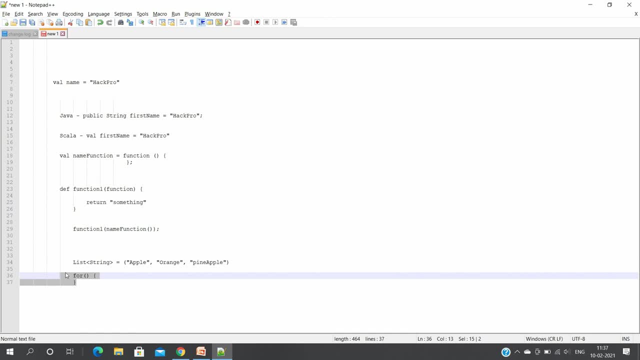 plays a major role. okay, that's what i'm trying to. i'm trying to tell, okay, um, yeah, um, next video we're going to see the uh setup of the how to do the local setup, and we can do some uh, some programs over there, some sample programs. 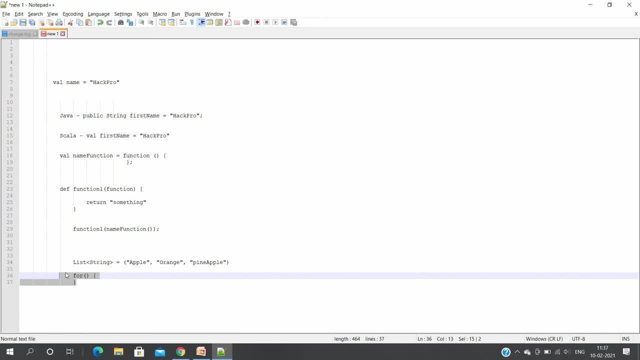 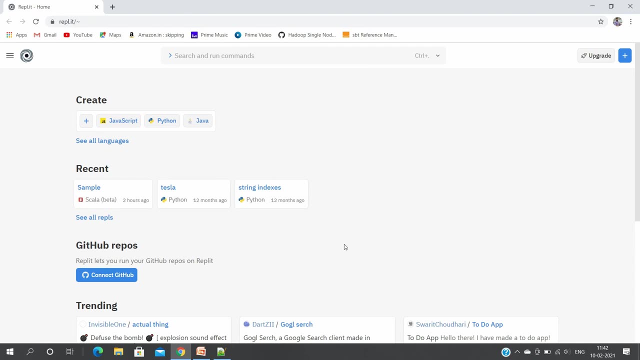 i can show you all these steps one by one. uh, thanks for watching the video. i know you people are eagerly waiting for the bonus tips here. it is okay, so you can directly go to the google and type ripple, so you will get this. uh, particular site rippleit. so this is the. 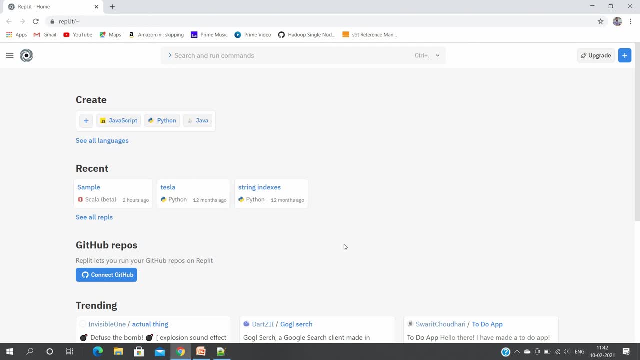 site. uh, i mean this is an online ide. you can do any stuff. so here, if you want to do some poc or uh, i mean just for testing, you can use this one. you can do any kind of language: java, scala, python, etc. okay, i just log in using my uh github account. if you have any other account like 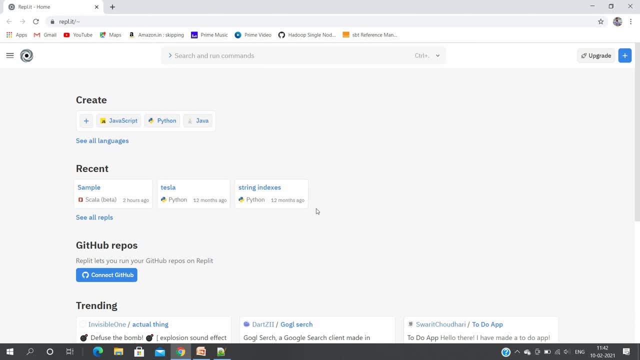 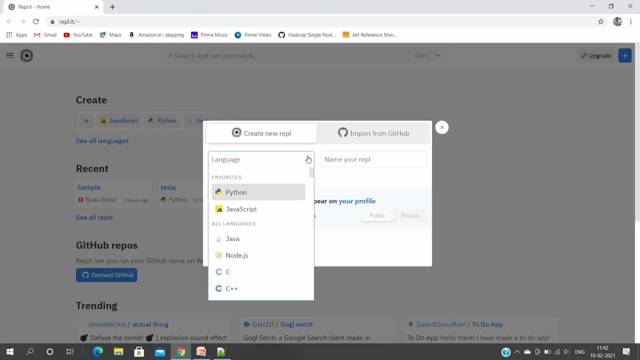 your gmail or anything, so you can use those accounts. okay, so what you can do, you can, you can create, uh, one, um, one ripple. okay, what i'm going to do, i'm going to see, if you see here, python, javascript, java, nodejs- there are a lot, of, lot of languages. okay, i'm going to take one. 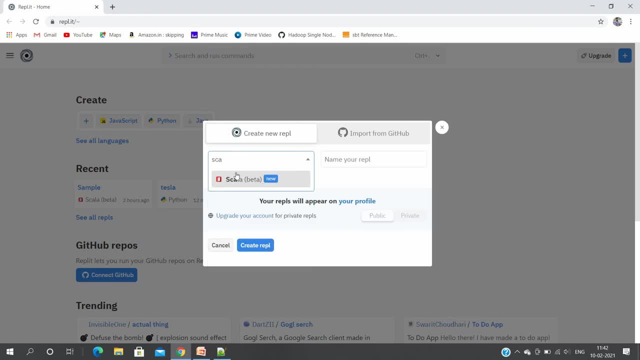 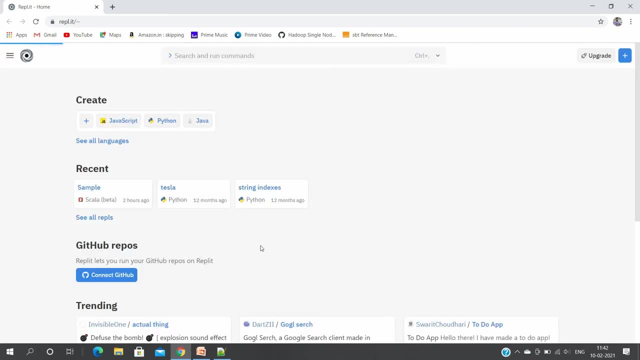 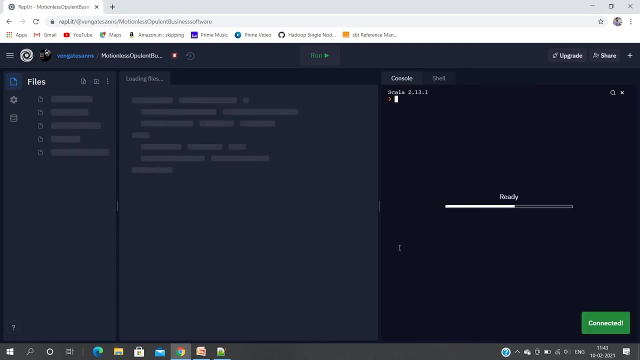 particular language, that is scala, scala, and you can give any name. i'm just giving as it is, i'm just creating it, so it's loading. uh, let it load. um, yeah, so if you don't have any id set up in your local, okay. for example, if you want to do, uh, some testing, okay, whether this code will work in this manner or 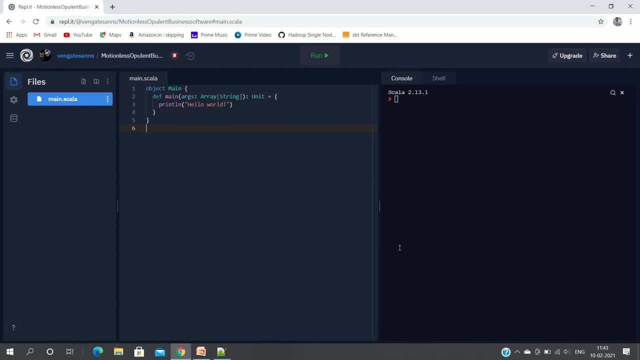 just some testing. you want to do so. for that you need to install ide and all those steps. instead of, you can directly go here and you can create a ripple and you can do: uh, see that main functions came and definition is there. you can directly uh, you can directly uh execute the here itself. so there, 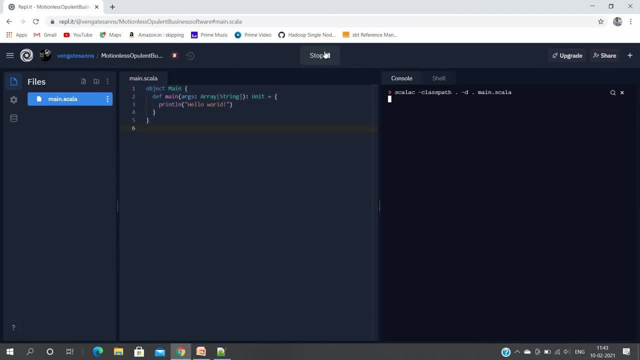 is one run button right. if i click on here, it will execute in the online itself. okay, this is uh, this will definitely helps you. i hope. i hope this will happen. definitely helps you people. so, um, let it compile. okay, i'll show this output and i can. 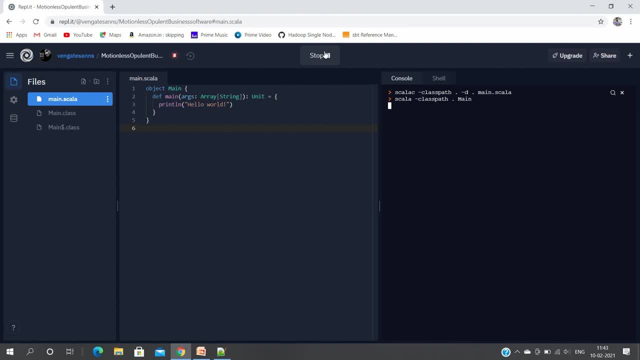 i can explain you. ah see, the hello world came, so printl. and they given the hello world, so hello world come. so don't worry about the- i mean uh programming syntax and all, but just think about the uh ripple and try to play around with that. um, i will see you in the next video. okay, thanks for watching the. video.